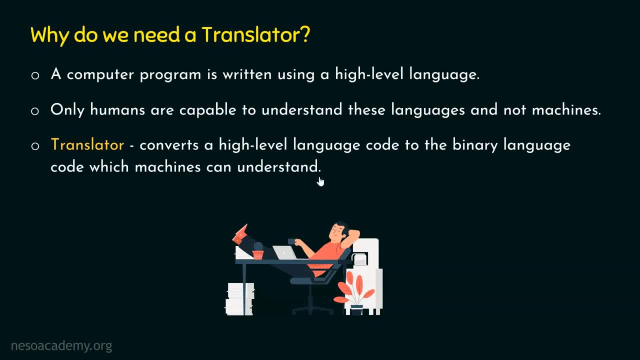 the binary language code which machines can understand. So the job of the translator is to convert a high-level programming language code, to convert a high-level language code to the binary language code which machines eventually can understand better. So we want our machines to understand the language, the things that we 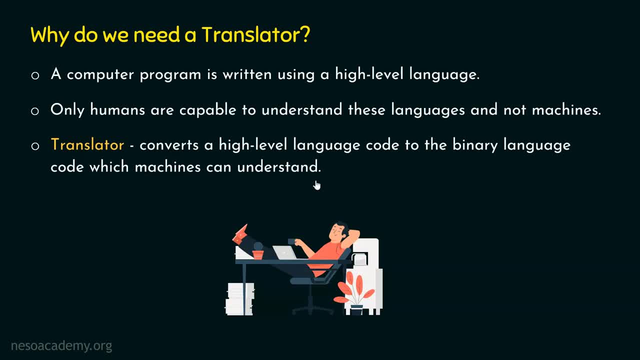 want them to convey. This is the reason we need a translator. As we know, machines cannot understand high-level language. We need a translator to convert the high-level language code to the binary language code which machines eventually can understand. So now you know why do we need. 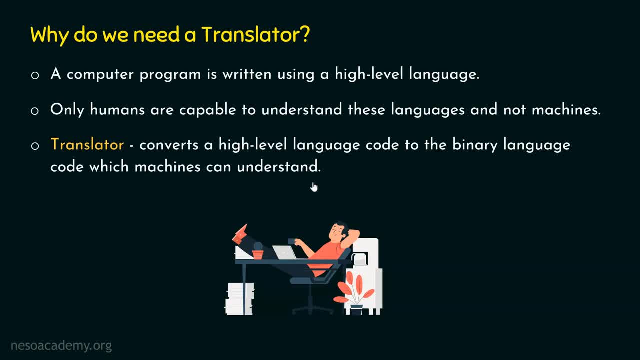 a translator. There is one more thing I would like to tell you. There are two types of translators. One is called compiler and the other one is called interpreter. In this presentation, we will try to understand what is a compiler. In the next presentation, we will understand what is an. 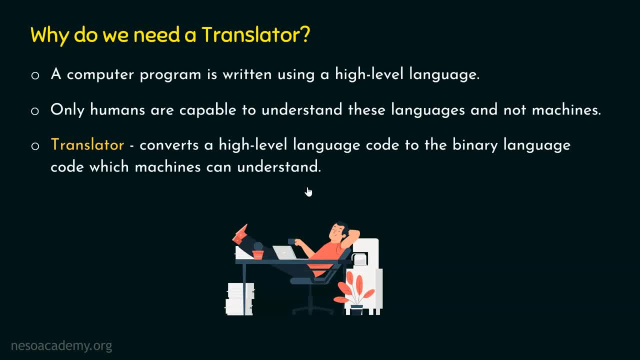 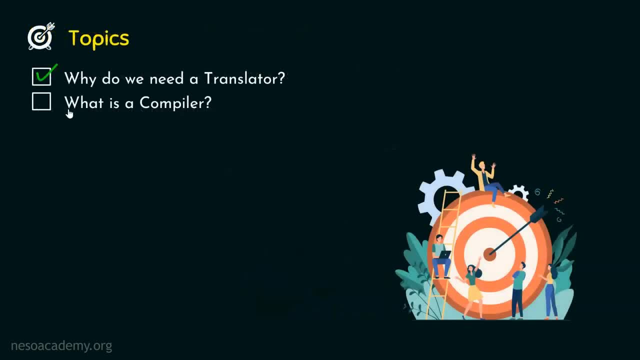 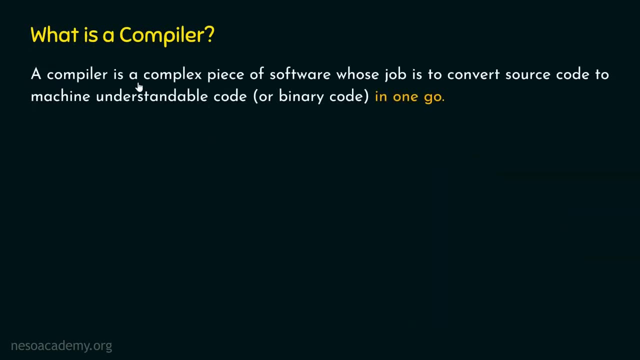 interpreter, and we will try to understand the differences between the two. We will understand these two topics in detail. First, in this presentation, we will try to understand what is a compiler. Now let's see what is a compiler. A compiler is a complex piece of software whose job is to convert source code to machine. 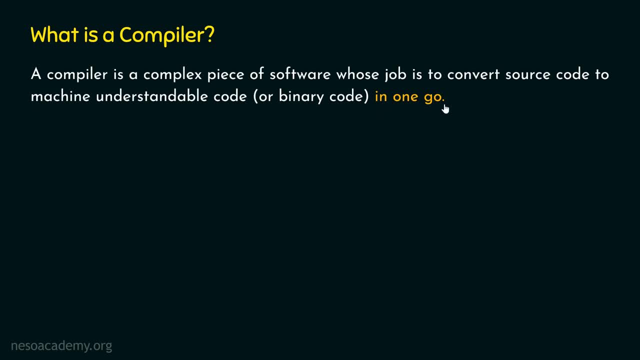 understandable code or binary code in one go. So a compiler is a piece of software. This is first thing. Many people have this confusion that compiler is a hardware. No, Compiler is a software and that too, a complex piece of software. It is very complex, It has a lot of 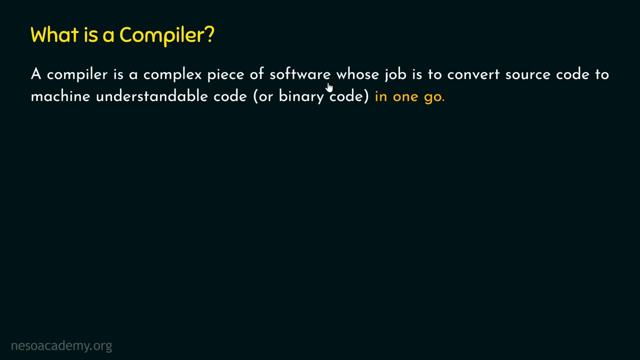 functionality. but the good thing is that we don't have to understand each and every detail about compiler, because understanding all those details is out of the scope of this course. A compiler is a complex piece of software whose job is to convert source code, that is, code we humans can. 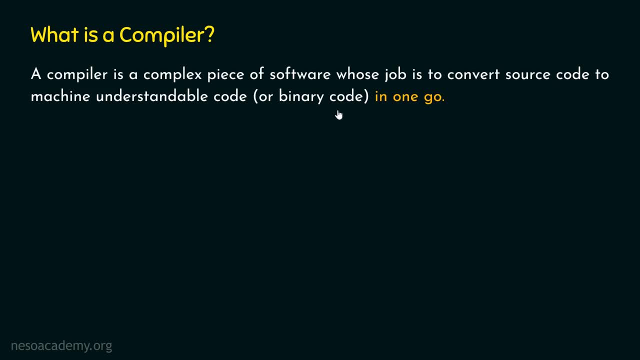 understand to machine understandable code or binary code. This means the code which machine can understand, So it converts source code to machine code in one go. Now, this is also important to understand, and in order to understand the meaning of this entire definition, I would like 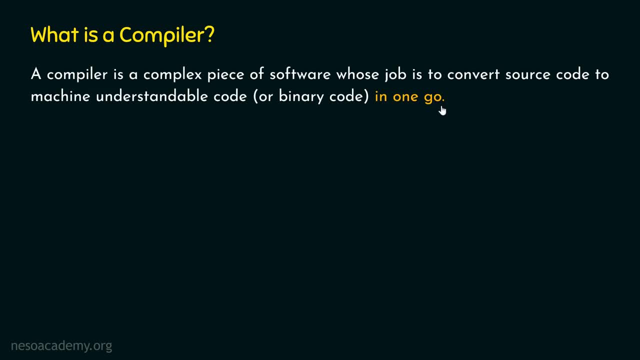 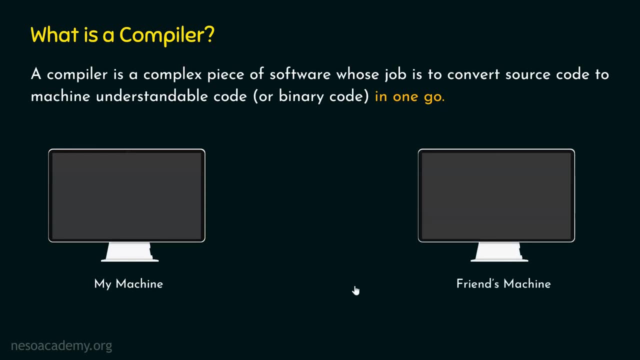 to give you one example to help demonstrate how compiler works. Let's say that this is my machine and this is my friend's machine. In my machine I have written this code, which is a C programming code. hash include stdioh int main. 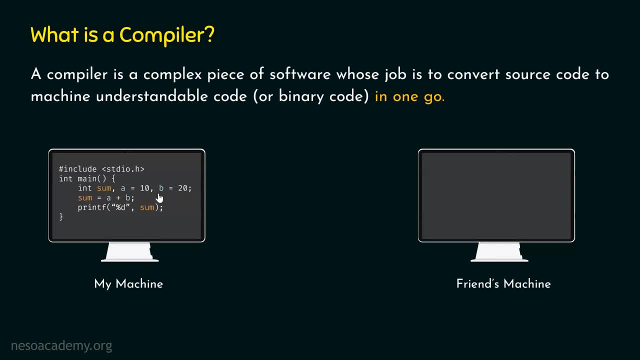 int, sum a equal to 10,, b equal to 20, sum equal to a plus b. and then I have a printf function which is used to print sum on the screen. Now, here I am trying to calculate the sum of a and b. 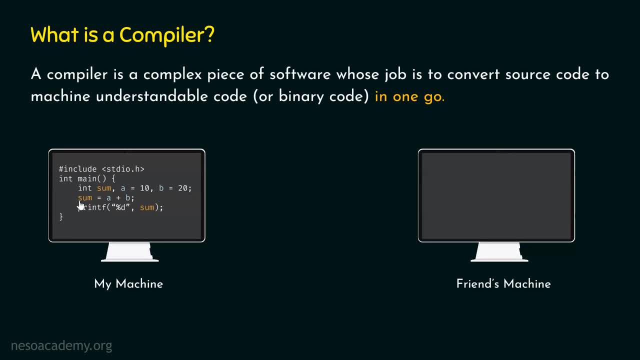 We know that a is 10 and b is 20, therefore the sum must be 30, because 10 plus 20 is 30. So eventually, I want to print sum on the screen, which means I want to print 30 on the screen. 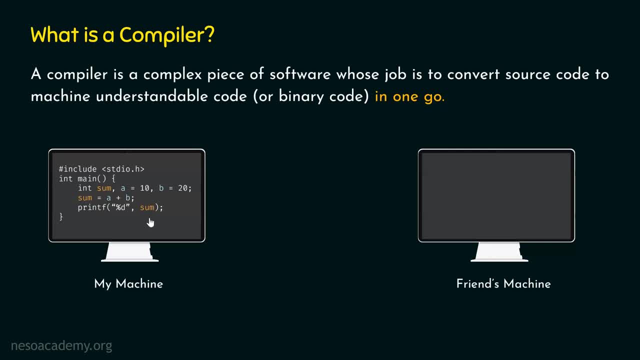 So with the help of this program, we will get the output 30.. Now you might be wondering: this course is all about Python, So why I took a C programming code? The reason is pretty simple. C programming language is a compiled programming. 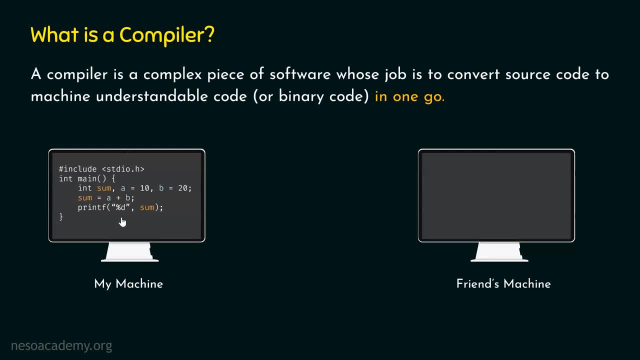 language. This means it uses compiler for its translation And as we are talking about compiler in this presentation, we need to consider a compiled programming language, and this is the reason why I took a C programming code. I hope now it is clear to you. 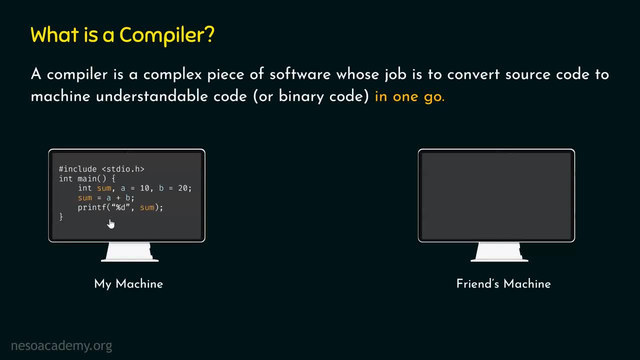 So I have written this C programming code and what I want to do now? I want to provide this code to compiler. This means I want to compile this code Before running this code. it is important to compile this code so that compiler will first translate this code to machine executable code. 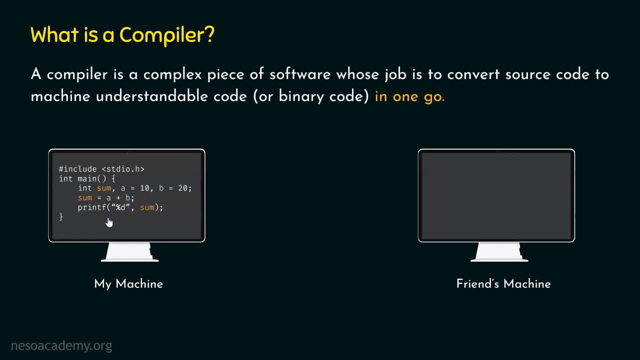 Eventually, that executable code will run on machine and machine will perform the task. That is what we want. So let's provide this code to the compiler and let's see what compiler will produce. If we provide this code to compiler, compiler in return will produce an. 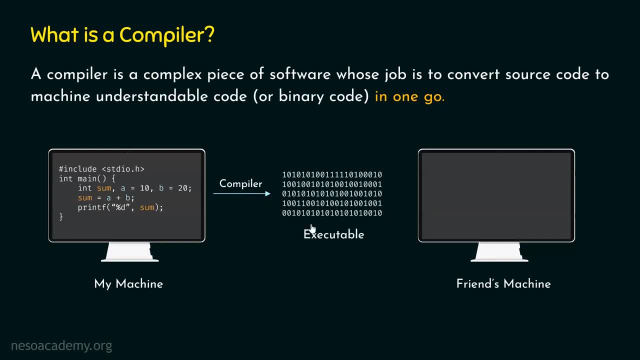 executable code. This code is called an executable code because we can directly run this code on our machine. We need to understand this: that this is called executable, and if my machine is a Windows machine, then my executable should have an extension: dot, exe. Understand this thing. 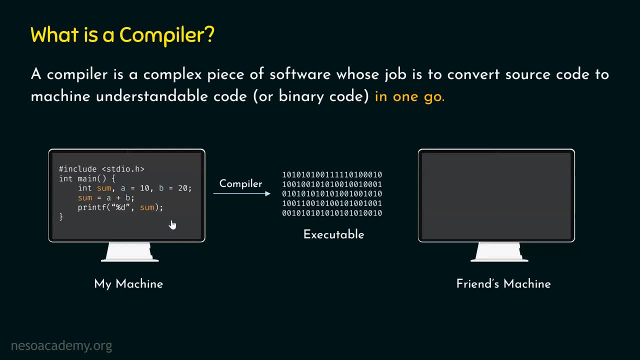 If I compile my code on Windows machine, then the executable must be having an extension: dot, exe. If, let's say, my machine is a Mac machine and if I compile this code on Mac machine, then I will get an executable with dot app extension. 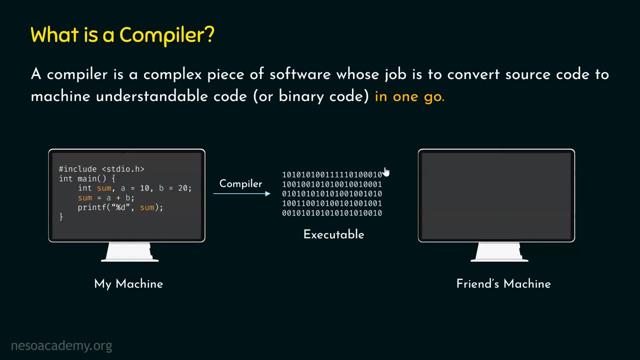 So extension matters, because this code is capable of running on Windows machines only if the extension is dot exe. If the extension is dot app, then the code is capable of running on Mac machine. So let's say that my machine is a Windows machine, then in that case the executable must have a dot exe extension. 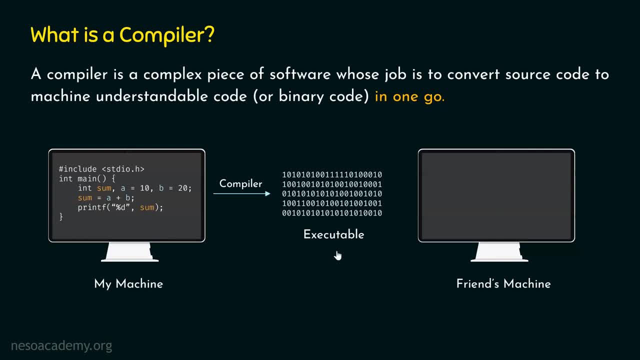 And this code is capable of running on Windows machines. only Now, let's say that my friend's machine is also a Windows machine. And what I'll do? I'll provide this code to my friend and I'll ask him to execute this code. 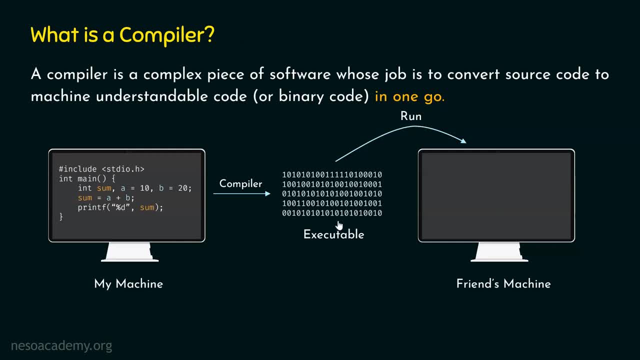 This means I want that my friend should run a Windows machine. Then after running this code, we'll get this output, that is 30.. Note this: that I have compiled the code in a different machine in my machine and we are running the code in a different machine. 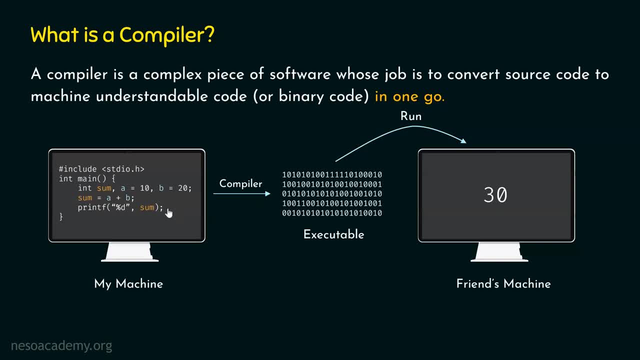 Compilation means that the code will get converted to executable And eventually we can provide this executable to any machine, and any machine is capable of running this code. Now, one thing that we need to remember is that if we compile the code on Windows machine, then we will get an executable with dot exe extension. 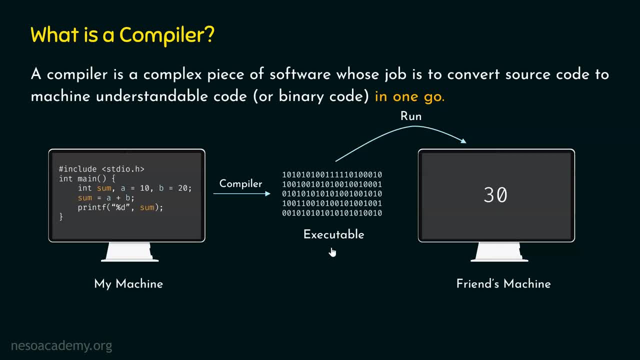 So note this: that this executable is capable of running on any Windows machine. I'm saying any Windows machine. My friend should have a Windows machine in order to run this code, And I'm assuming this, that my friend's machine is also a Windows machine. 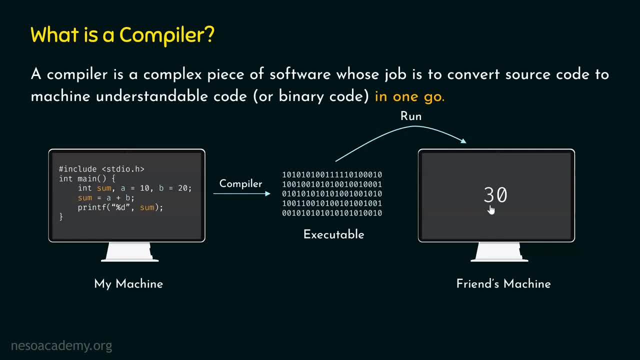 So he can run this code And after running the code he will get this output, that is 30.. I hope now it is clear to you. Now I would like to take you to the IDE or Integrated Development Environment, where we will compile this code and we will see the executable. 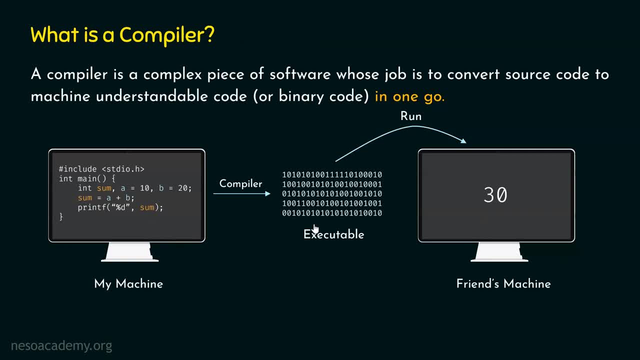 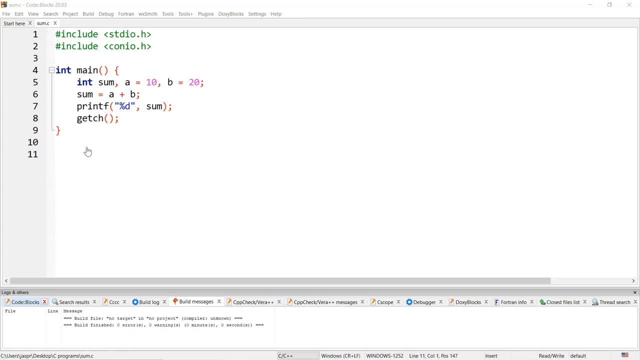 Precisely. I will take you to the CodeBlocks IDE, where we will compile this C program. So let's move to the CodeBlocks IDE. Now we are in CodeBlocks IDE and you can observe the same C program and the file name is sumc. 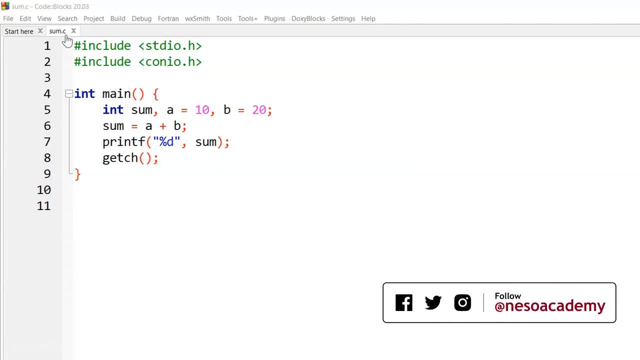 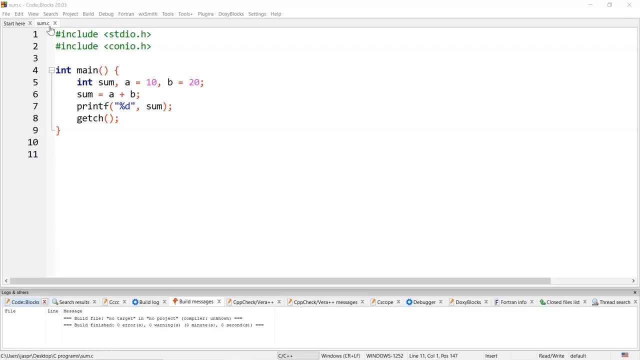 Now this file is available in C programs folder And I want to show that C programs folder to you. So let me take you to that C programs folder, which is available in my desktop. Now we are in my desktop and here we have the C programs folder. 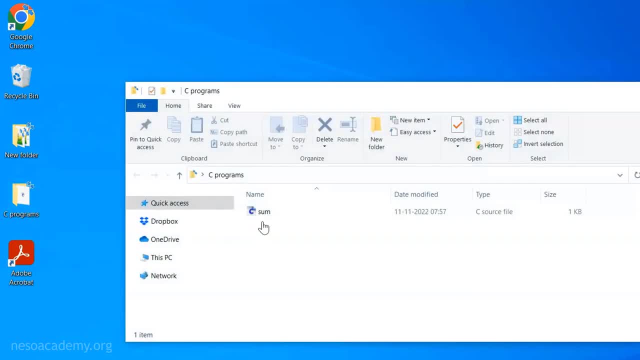 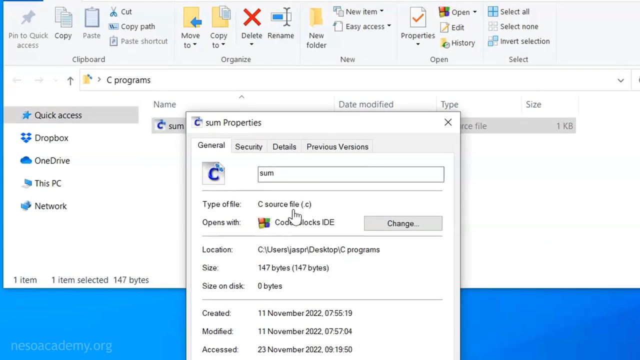 Let's open this folder. In this folder we have the sumc file. We can always check the extension of this file by right clicking on this and then clicking on properties. You can observe this is C source file And the extension is c. 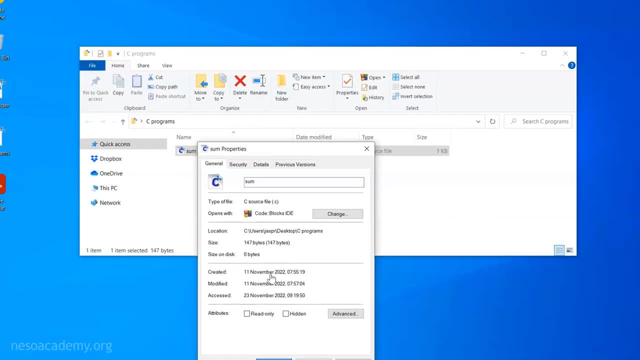 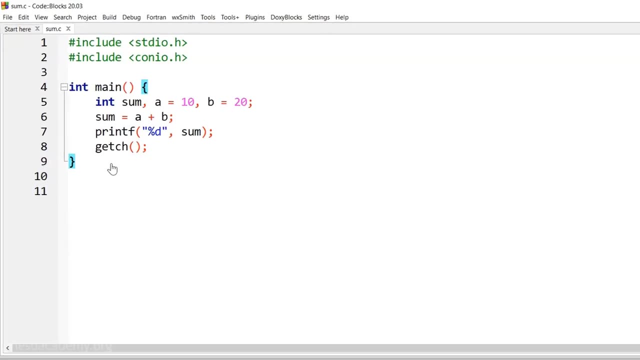 This is the same file where we have our C program. Let's click on OK And let's get back to our IDE. You might have observed this already, that in this C program I have added two lines: hash include conioh and getch. 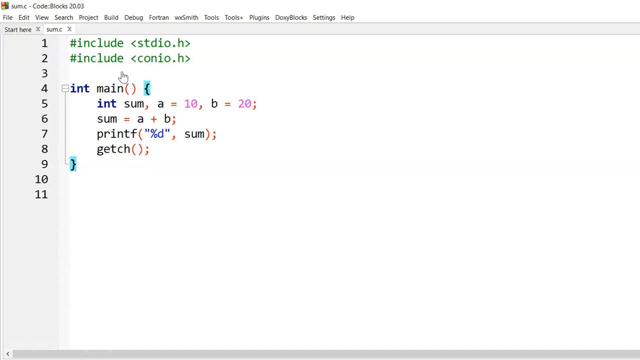 Getch function is needed, and for this I need to include this header file, conioh, because getch function is available in this header file only Now. this getch function is needed to hold the screen of the executable. After compiling this code, we will get an executable. 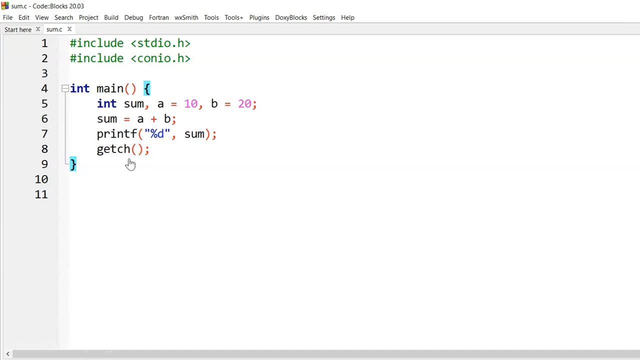 We know this already Now: that executable will get stored in the same folder where this sumc is stored, That is, we will get an executable in C programs folder If we double click on that executable. this means if we run that executable. 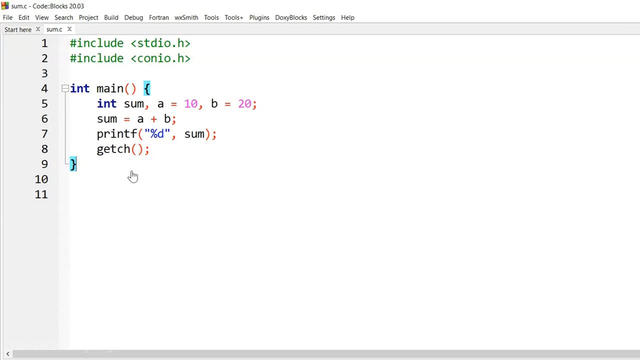 we would be able to run that executable. We would be able to see the screen of the executable only for few seconds and then it will go away. In order to hold the screen, we need this getch function. Getch means get character. This function allows user to enter the character on the screen that is, on the executable screen. 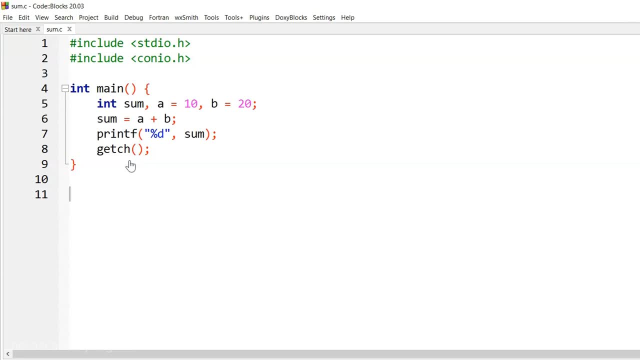 So this function holds the screen until user enters a character. Now, it could be any character, It could be enter also. So it depends on the executable, It depends upon the user. You will see in a moment that how we can run that executable and we will observe a blinking cursor. 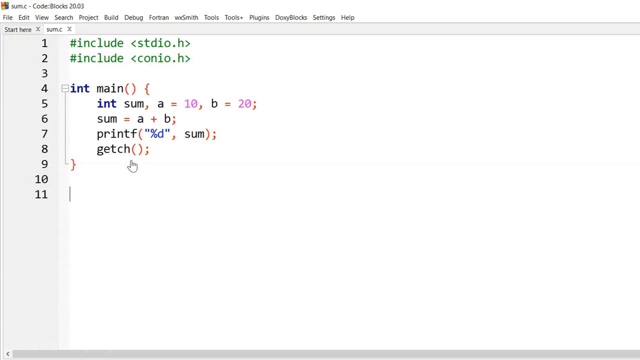 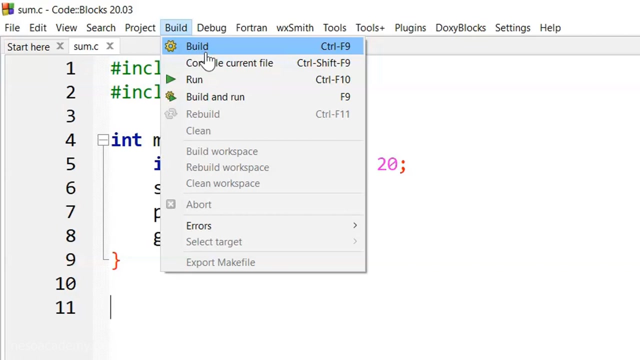 which asks us to enter some character. So now let's compile this code and let's see whether the executable is available in the same folder or not. Let's click on this build. We need to click this build. Build means compile, Okay. 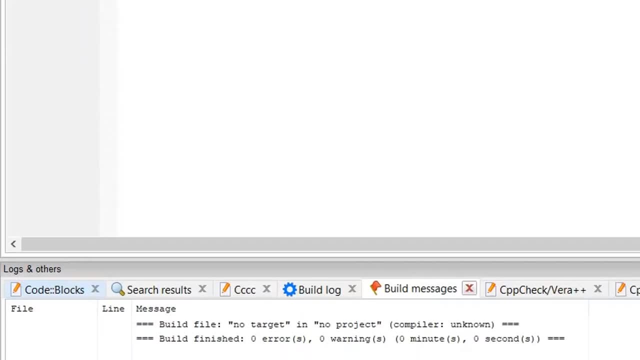 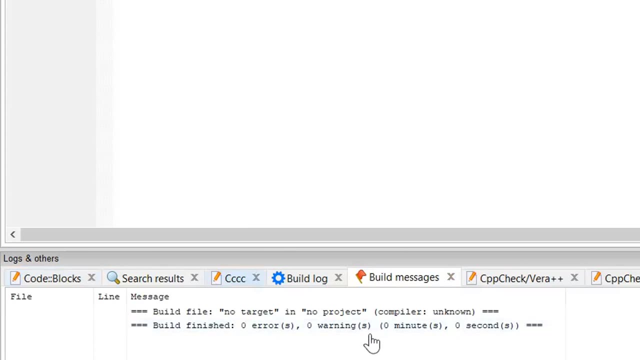 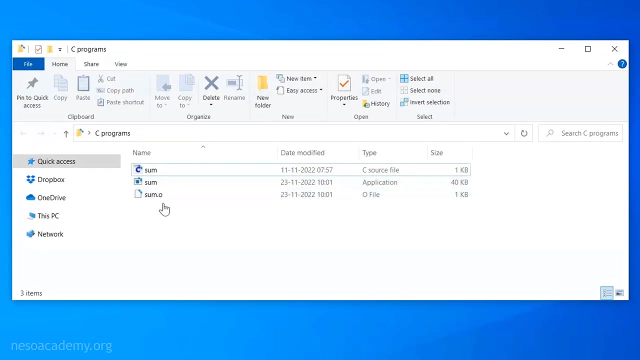 So let's click on this build Now. the build is successful, which means compilation is successful. There is no error, as you can observe: Zero errors, zero warnings. Now let's get back to the same folder. You can observe that there are two more files in this folder. 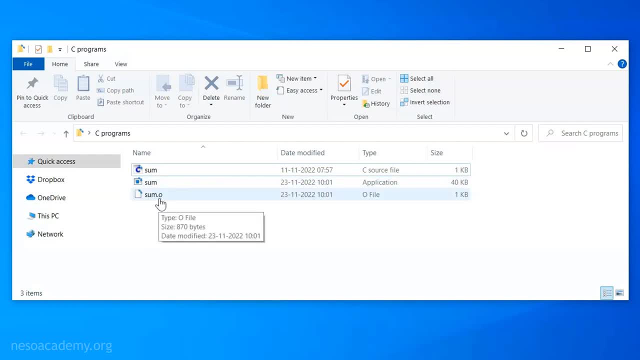 This is sumexe file and this is sumo file. This file is an object file and we don't have to worry about this at this moment. What we need to consider at this moment is this sumexe file. This is our executable, which we can run on any Windows machine. 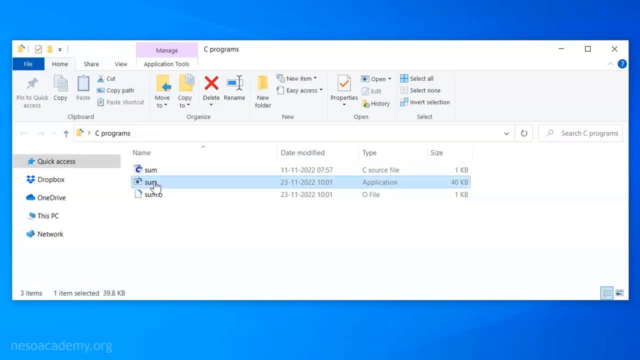 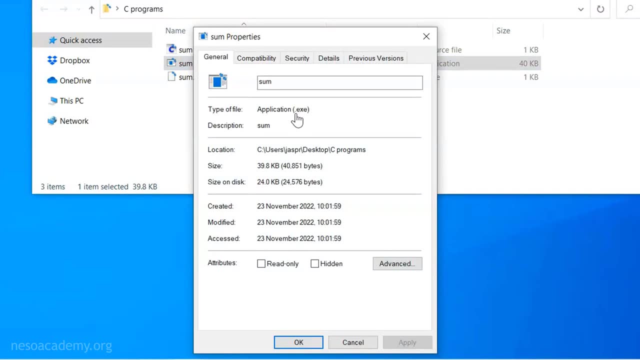 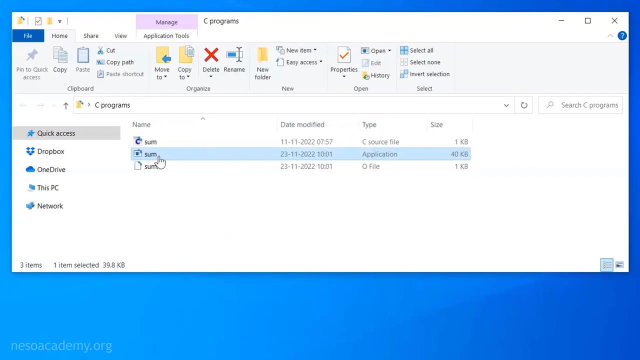 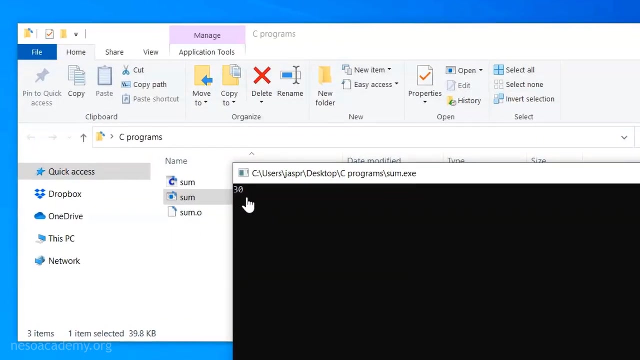 You can check the extension of this file by right clicking on this and then clicking on properties. Here we can observe that this file has extension dot exe. Let's click on ok. and now let's run this file by double clicking it. You can observe the output is 30 and there is one blinking cursor here. 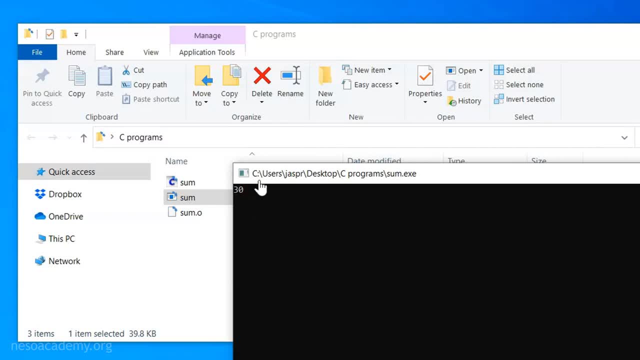 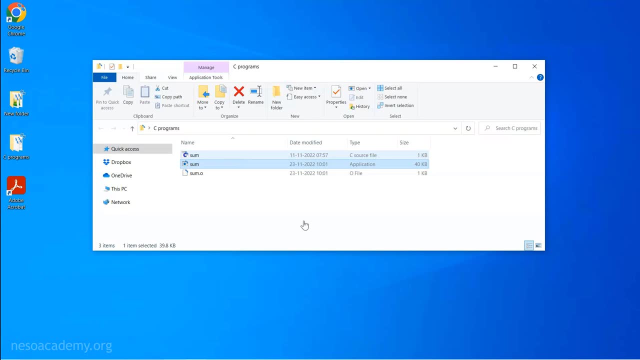 It is asking a character from us. Let's say I provided it a character. h Observe that the screen is closed. So after providing the character, the executable will go away. So in this way we can run our executable and we can provide this executable to any Windows machine. 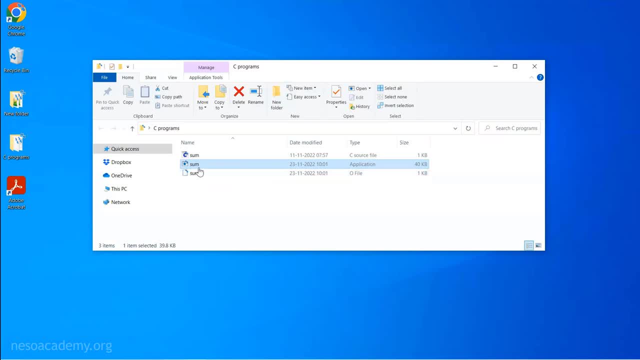 Now, any Windows machine is capable of running this executable. I can provide this executable to my friend, as my friend has Windows machine, So he can run this executable without the need of this c file. Now, he will not compile this file. 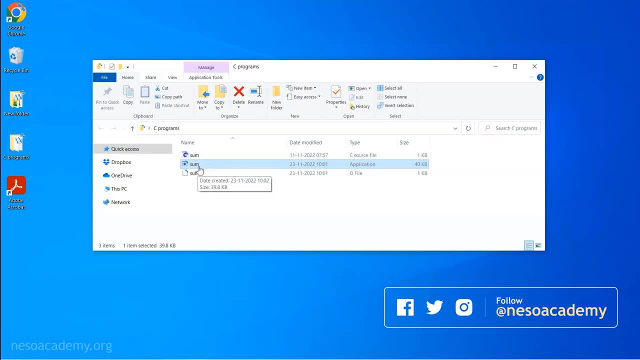 He will just use this executable and run this After compilation. we now know that we will always get an executable and that executable is capable of running on any Windows machine. Remember that I have compiled this sumc file in my Windows machine. This is the reason why I am getting a c file.